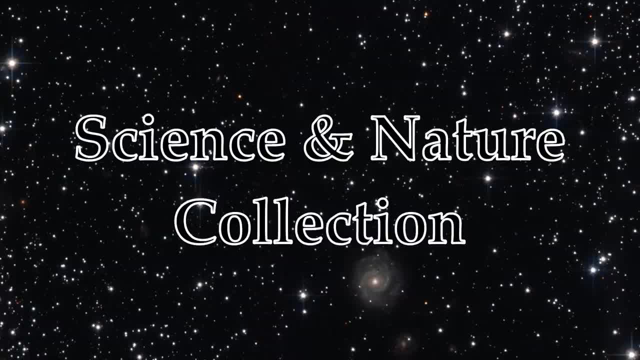 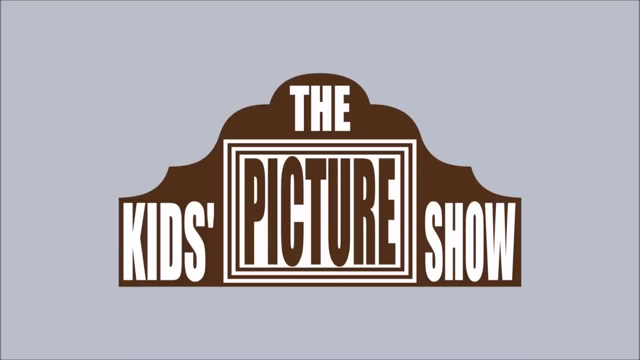 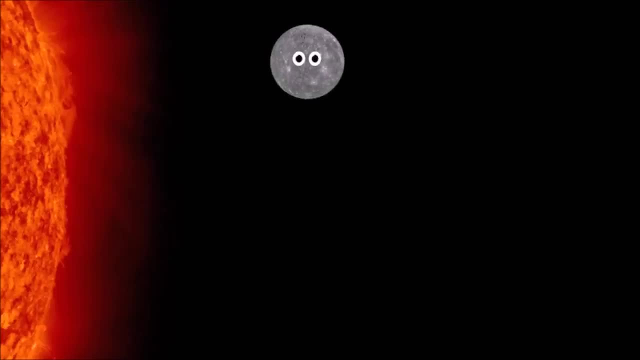 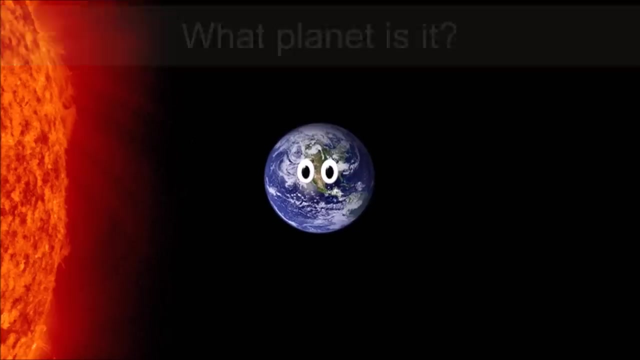 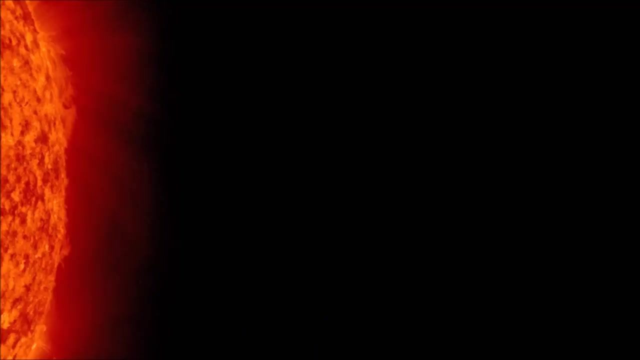 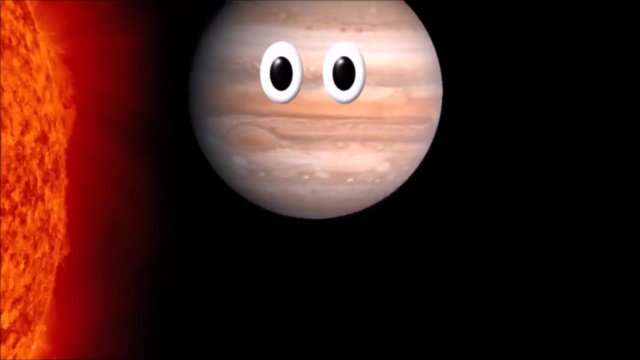 Science and Nature Collection. What planet is it? What planet is it? It's Mercury. What planet is it? It's Venus. What planet is it? It's Earth. What planet is it? What planet is it? It's Mars? What planet is it? 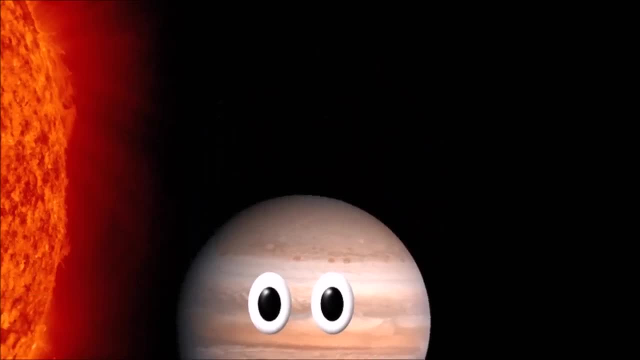 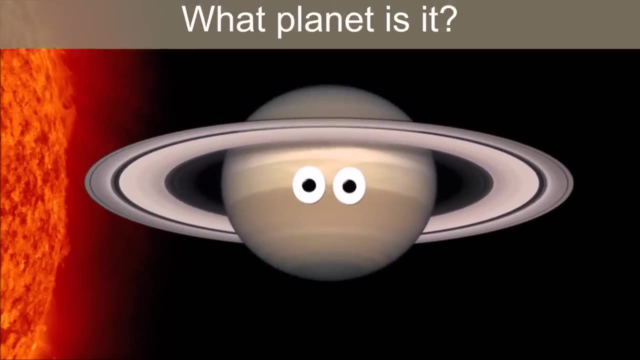 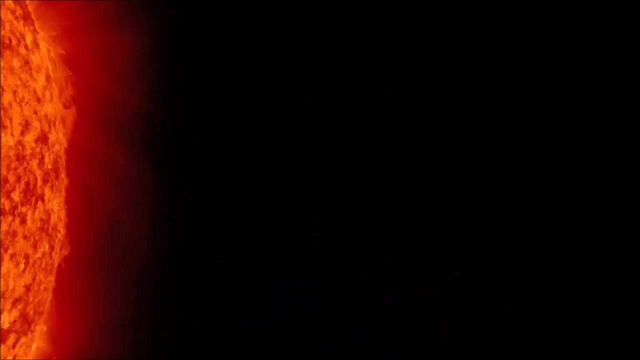 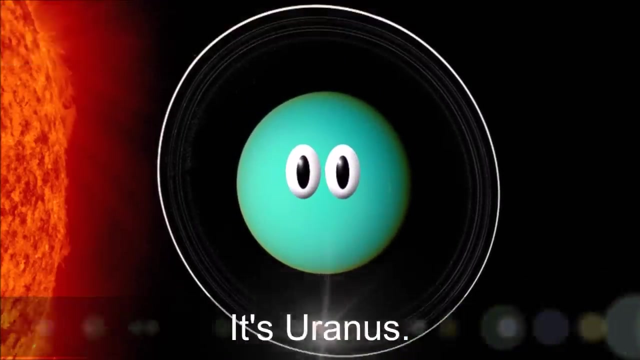 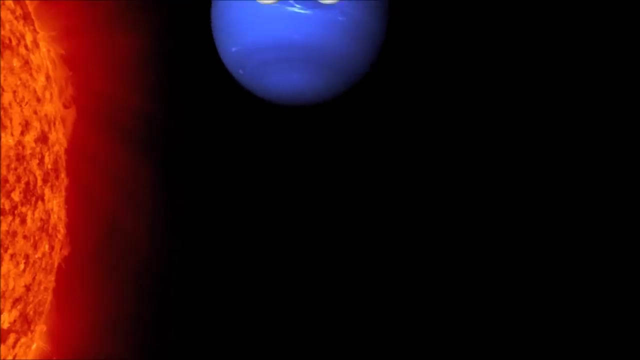 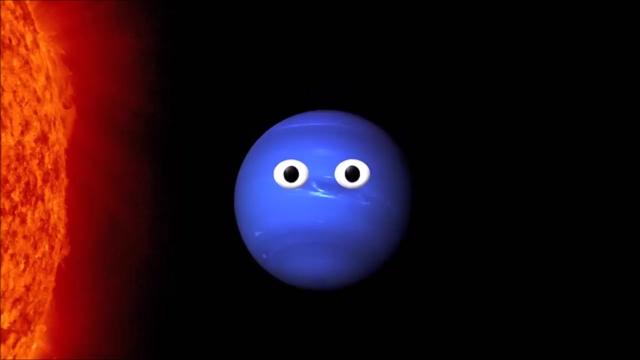 It's Jupiter. What planet is it? What planet is it? It's Saturn? What planet is it? It's Uranus. What planet is it? It's Neptune. What planet is it? It's Pluto. What planet is it? 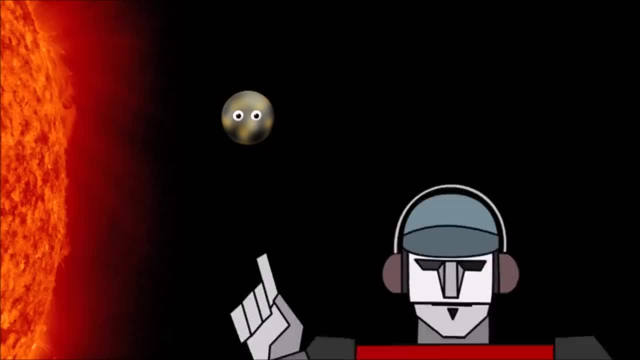 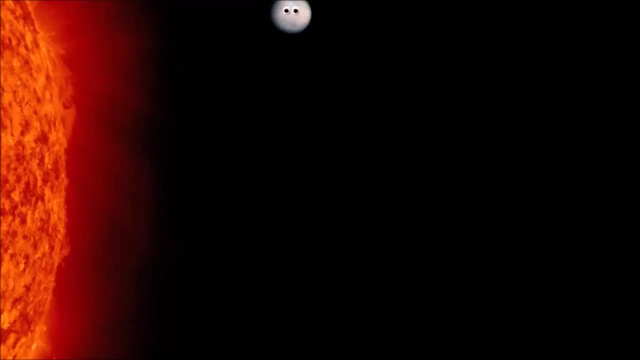 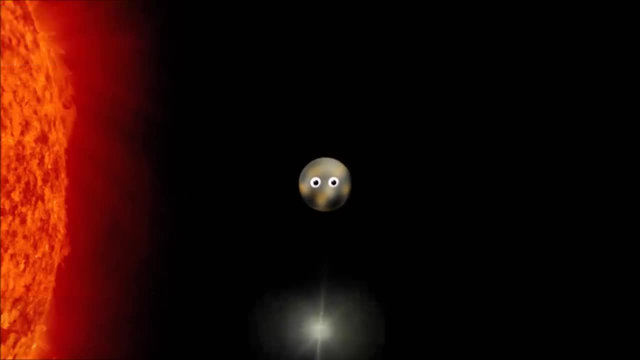 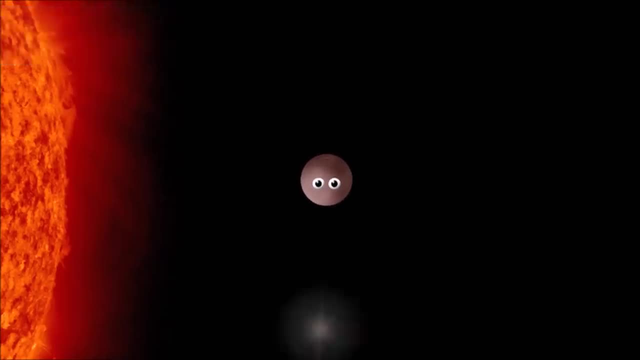 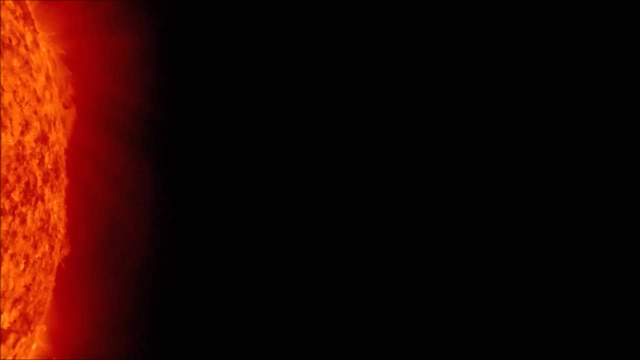 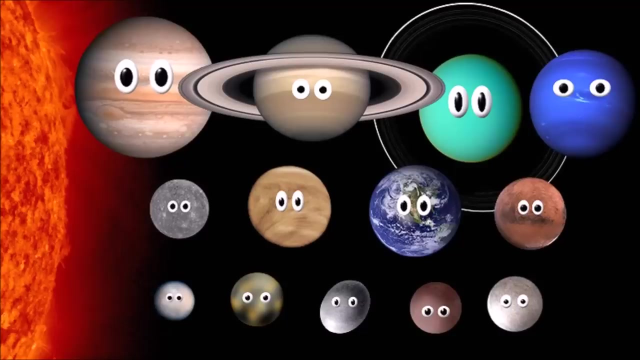 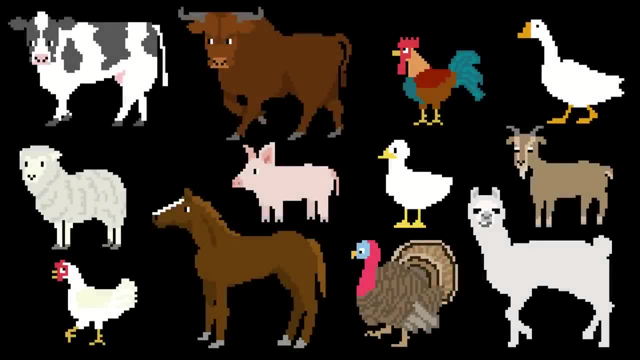 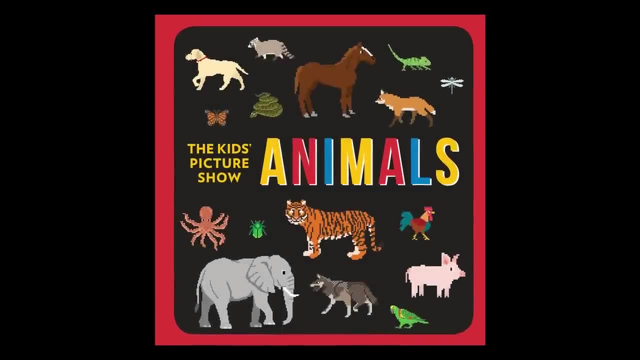 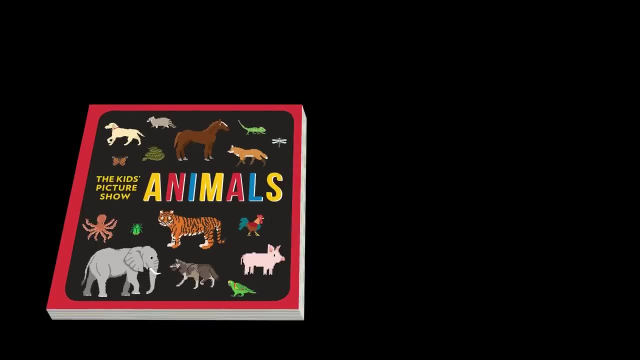 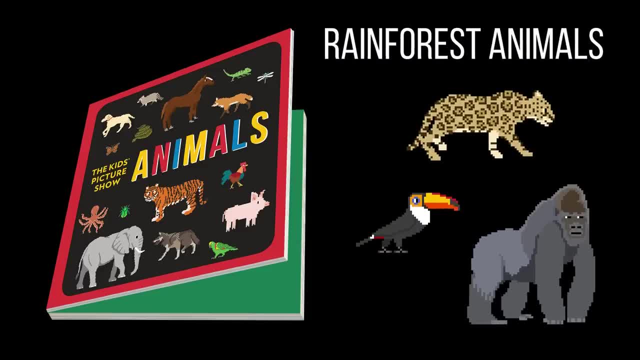 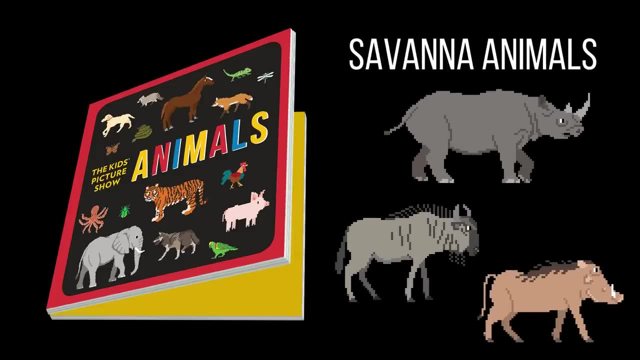 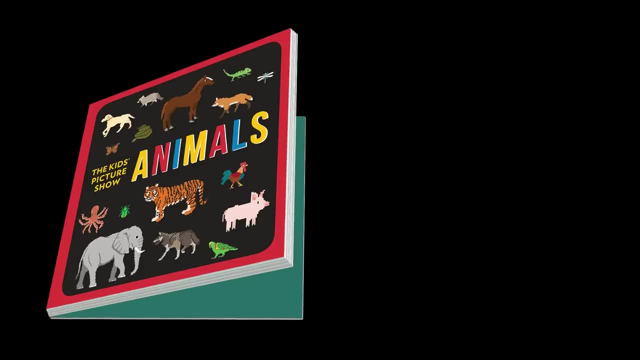 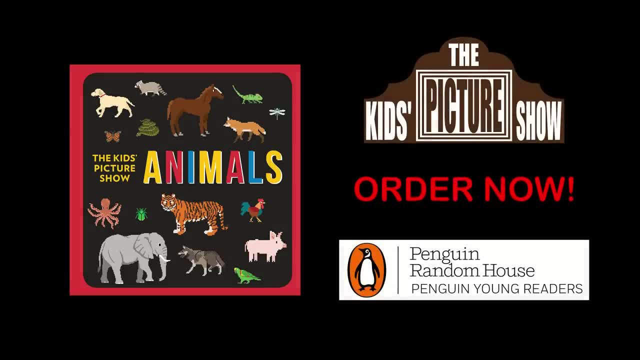 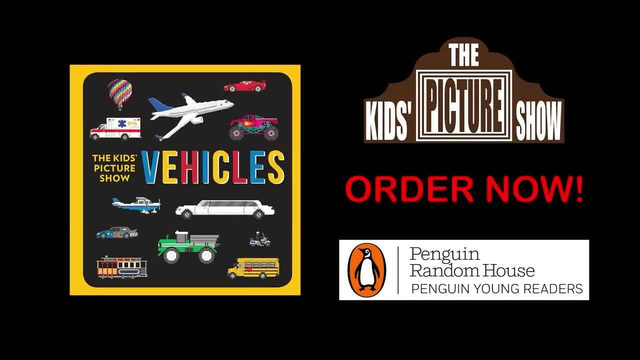 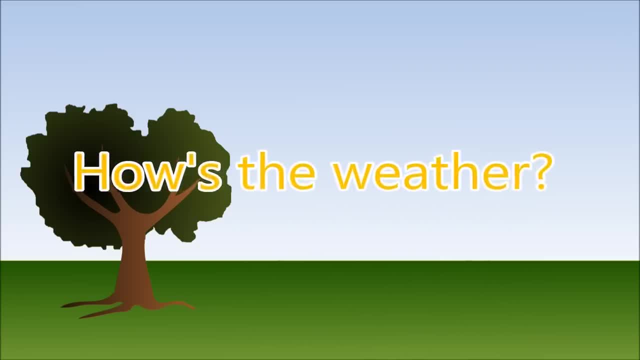 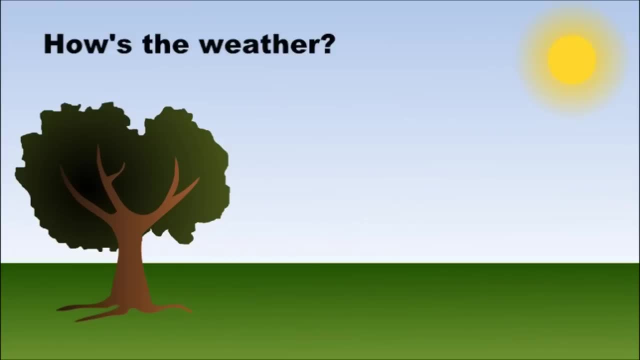 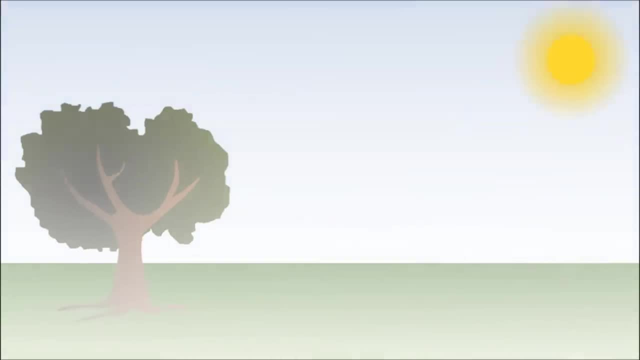 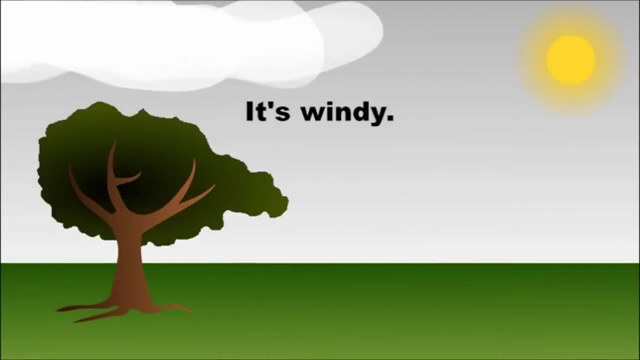 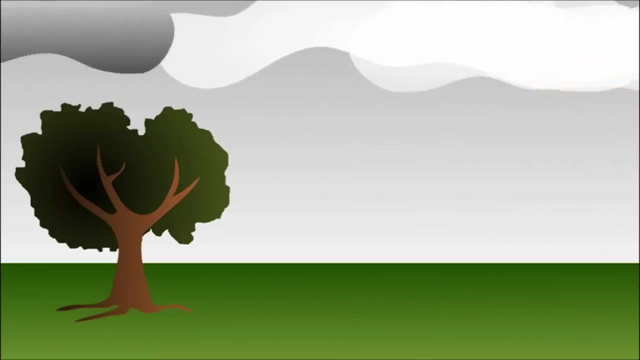 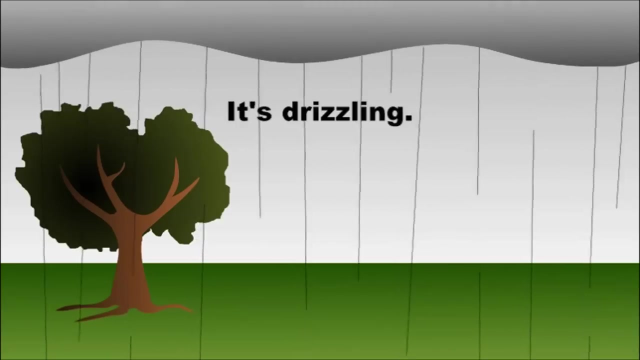 It's cold. How's the weather? It's foggy, It's cool. How's the weather? It's windy, It's partly cloudy. It's cloudy, It's sunny. How's the weather? It's drizzling, It's raining. 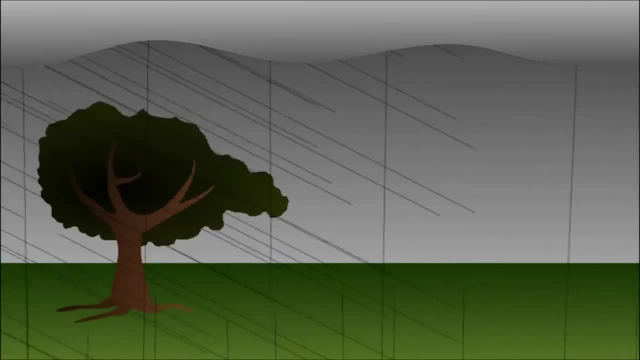 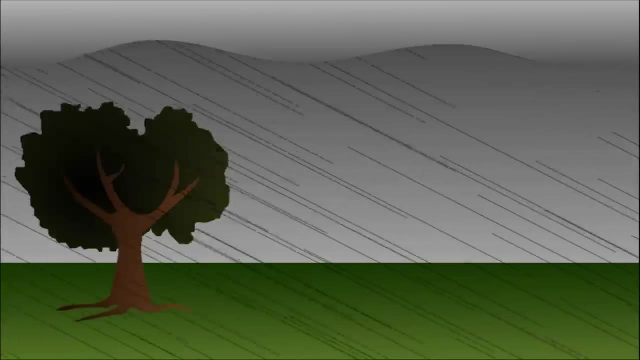 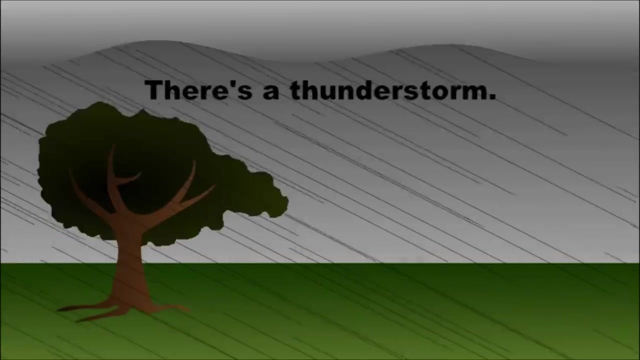 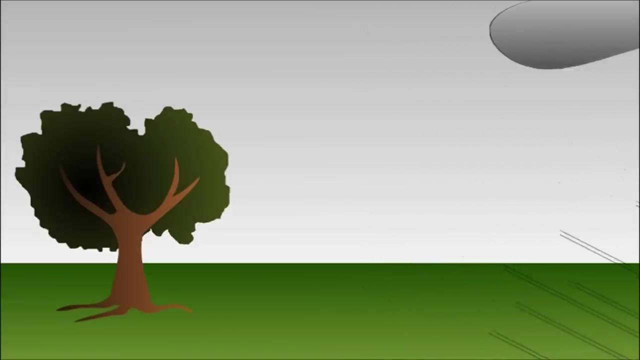 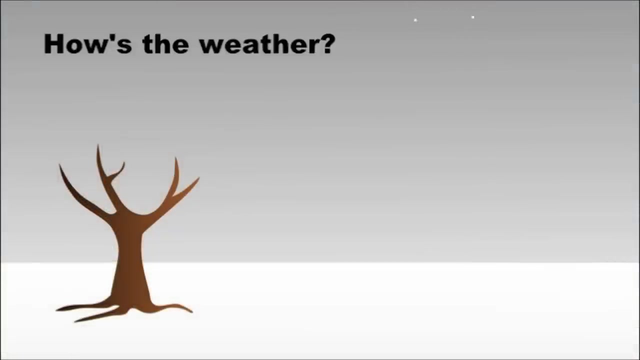 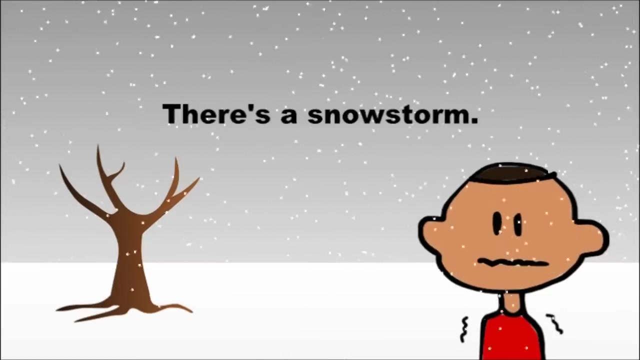 There's a downpour. How's the weather? It's stormy. There's thunder and lightning. There's a thunderstorm. How's the weather? It's snowing. It's cold. There's a snowstorm. There's a blizzard. 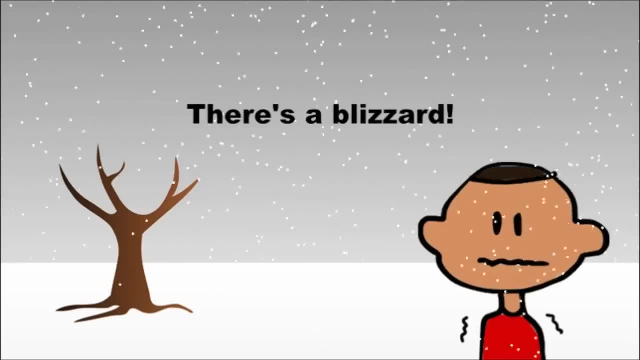 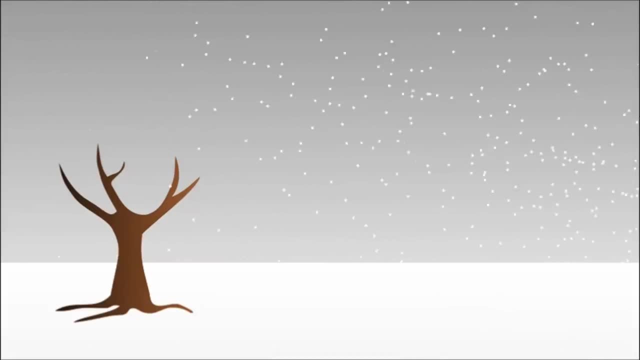 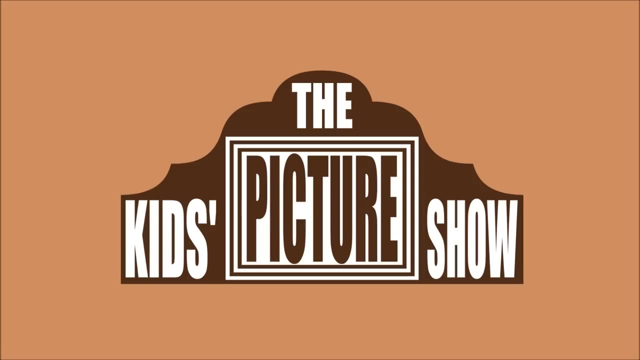 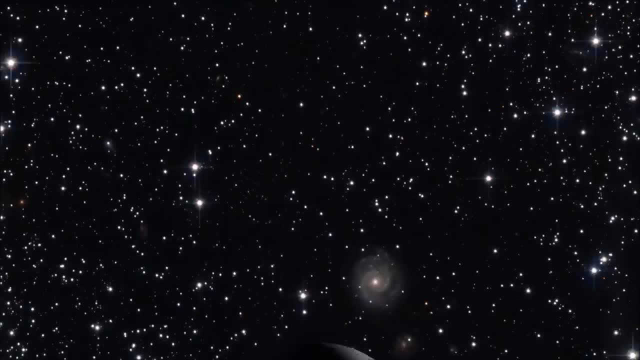 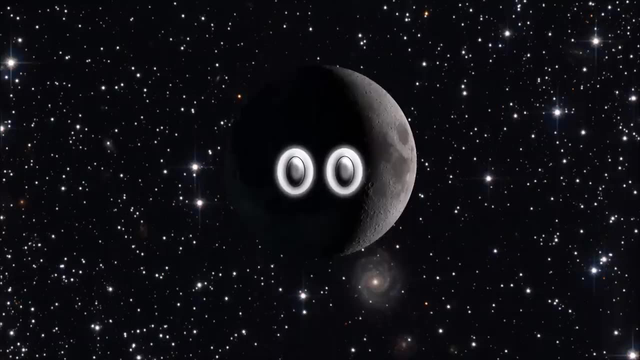 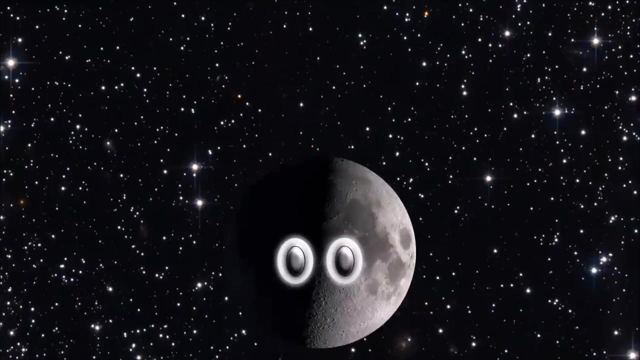 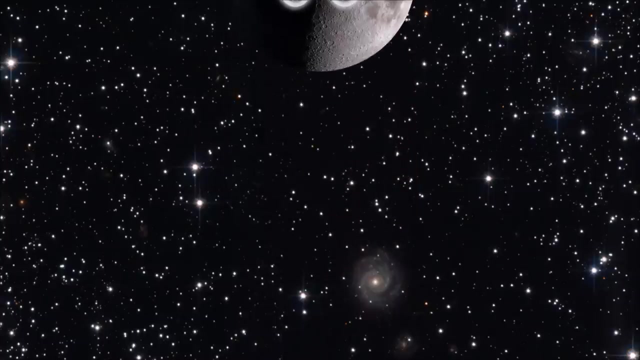 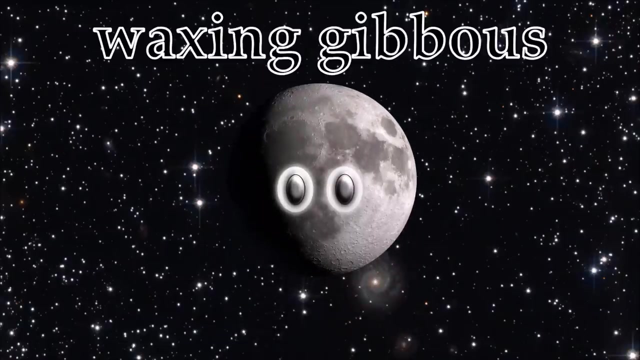 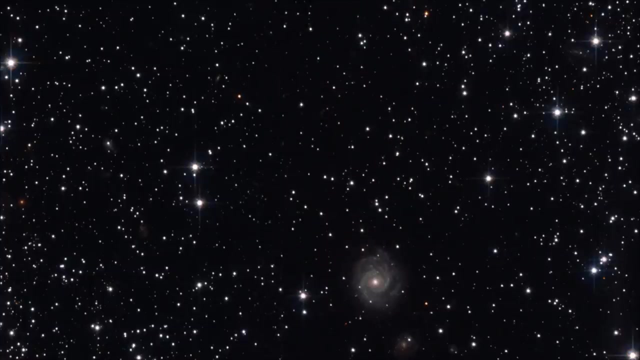 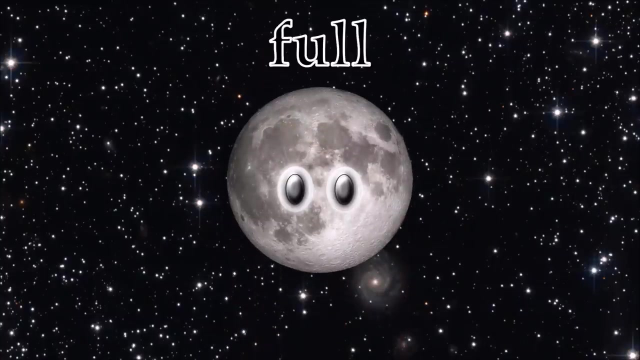 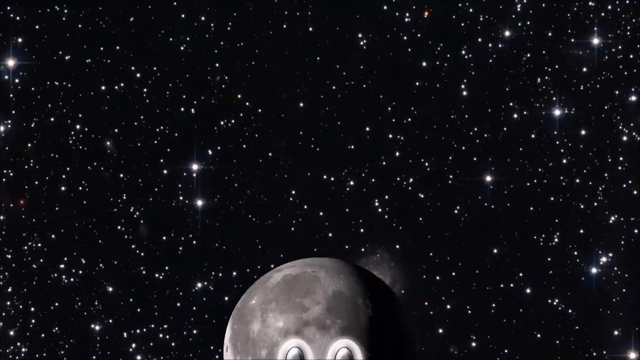 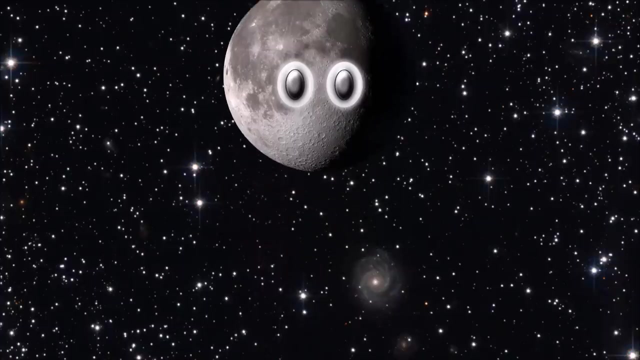 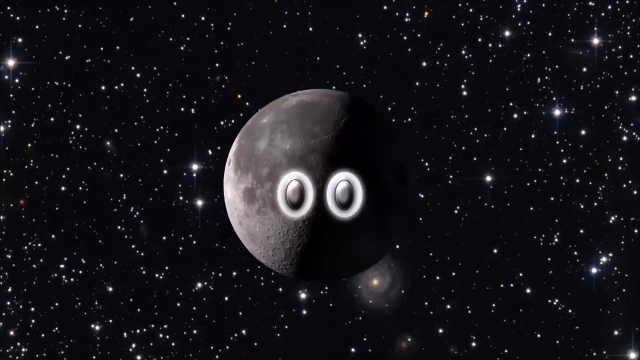 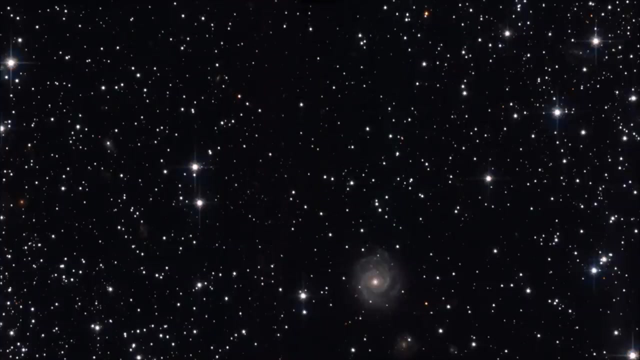 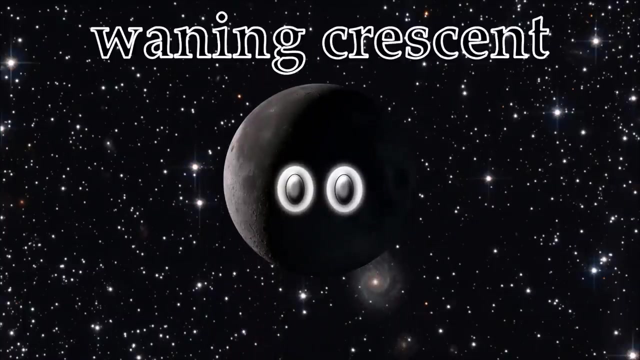 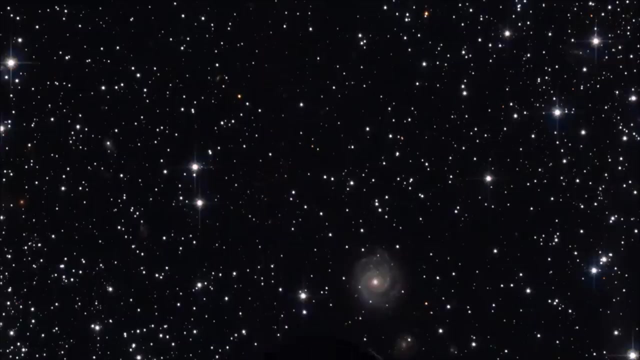 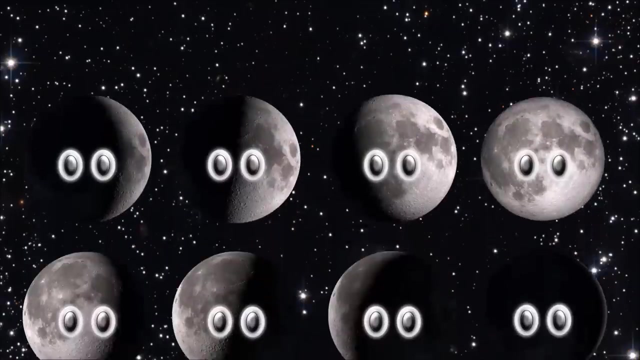 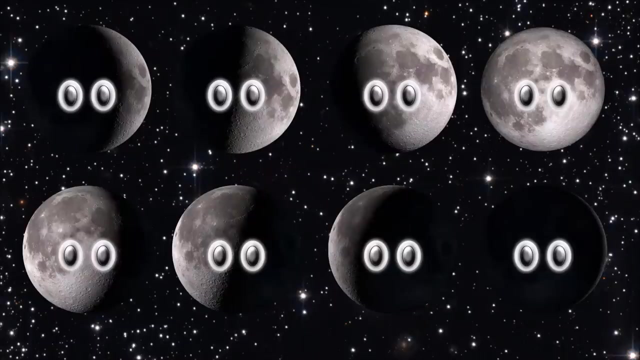 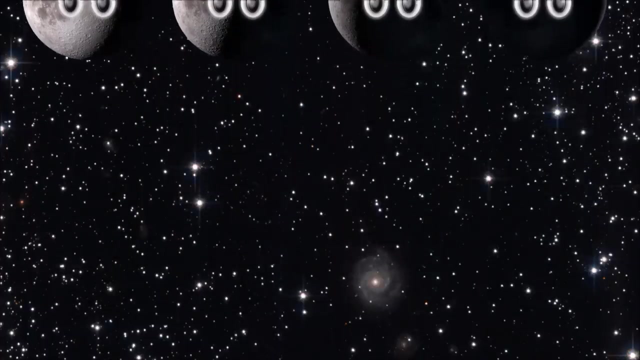 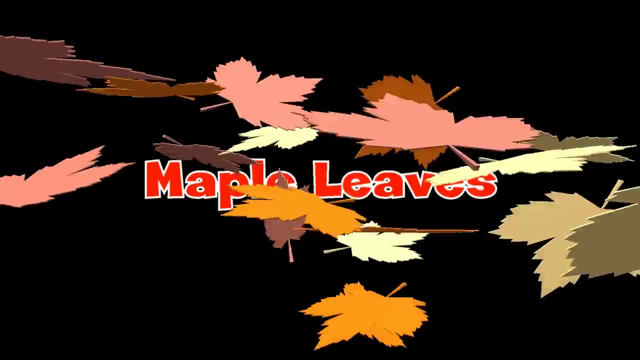 Phases of the Moon: Waxing Crescent- First Quarter Waxing- gibbous- Full Waning- gibbous- Third quarter Waning- crescent- New, New. Keep watching for more, For Maple Leaves, Maple Leaves. 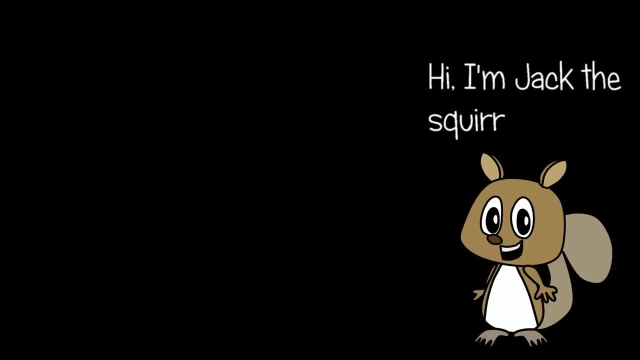 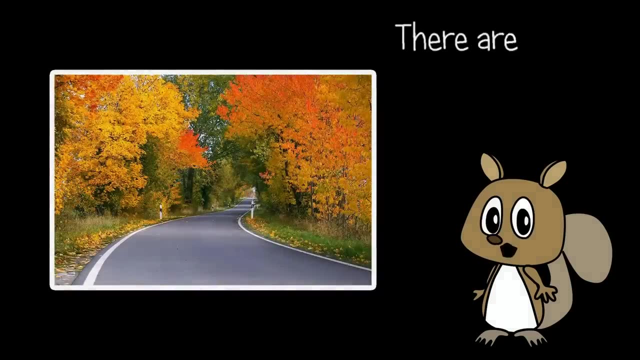 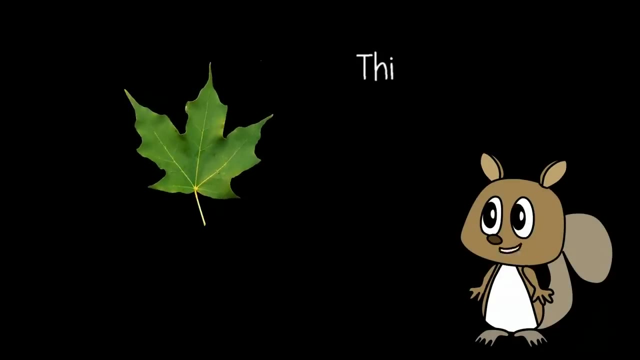 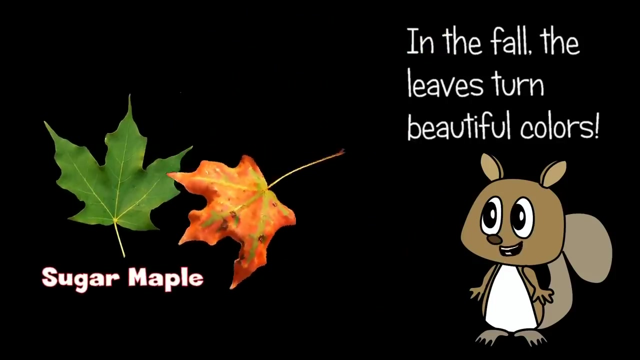 Hi, I'm Jack the Squirrel. Do you like Maple Leaves? There are many different kinds. Let me show you. This is a sugar maple. This is a sugar maple leaf. It has five pointy lobes. In the fall, the leaves turn beautiful colors. 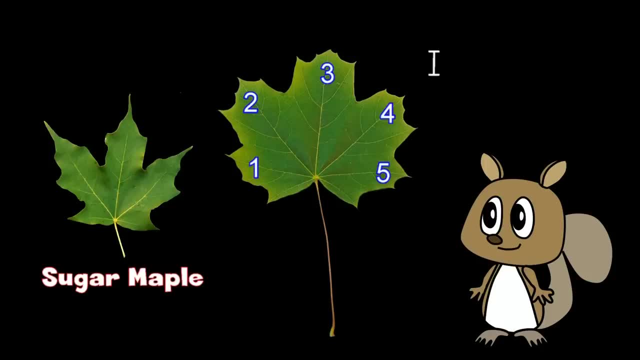 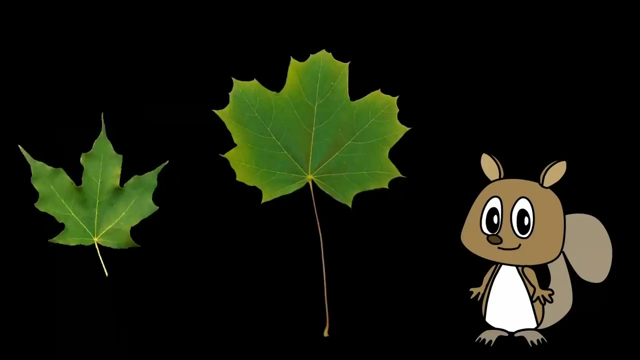 What's this one? It also has five pointy lobes, But it's bigger and wider. It's a normal maple leaf. It's a Norway maple leaf. Check the tips of the leaves. Check the tips of the leaves. Norway Maple Leaves have sharp tips. 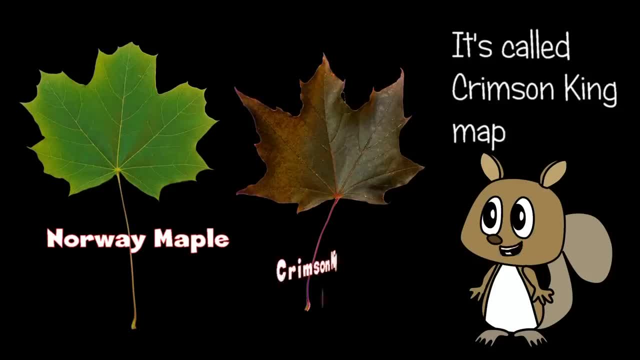 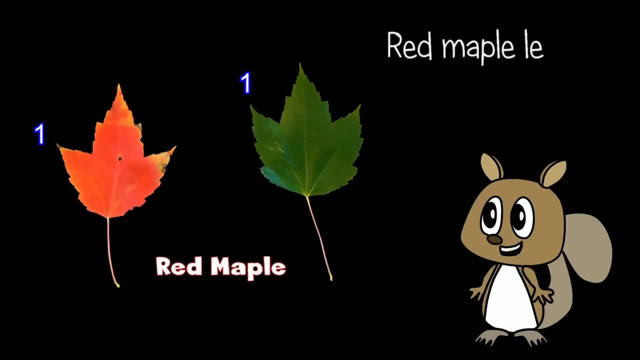 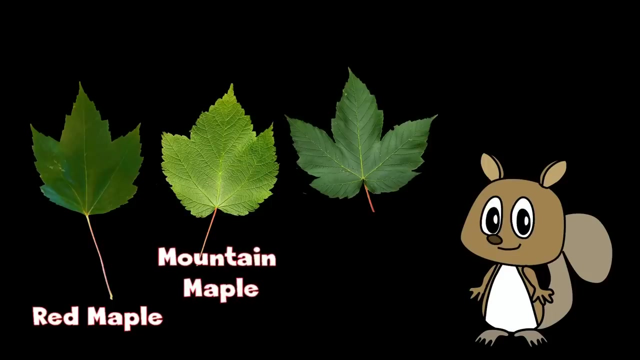 This is a kind of Norway maple with red leaves. It's called Crimson King Maple. It's called Crimson King Maple. Red maple leaves have three shaggy lobes. some leaves have small lobes here. Here are two more similar leaves. They're all shaggy. 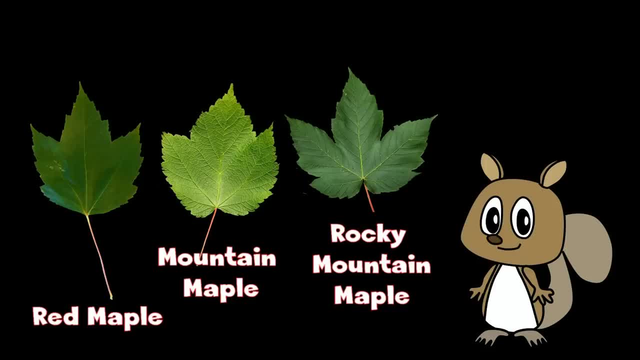 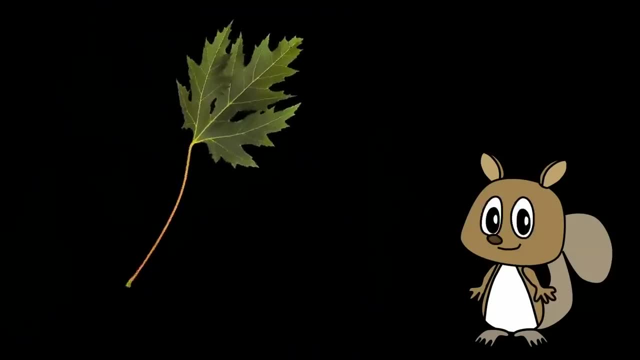 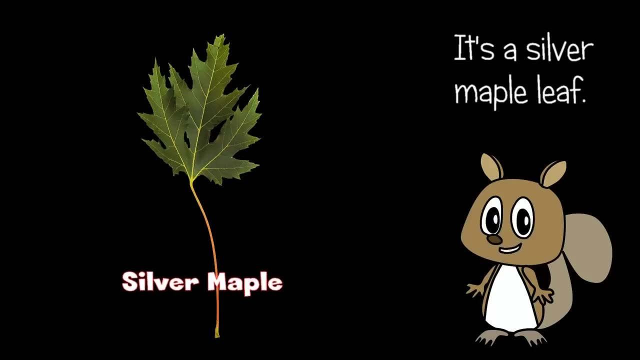 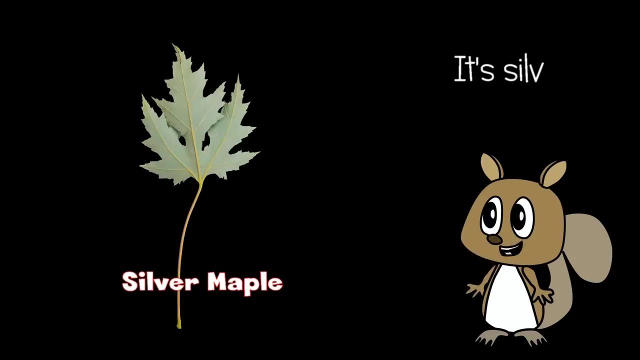 But not the same. Mountain maple leaves have textured veins And they're a little bit rough. Wow, this one looks cool. It's a silver maple leaf. Check out the back: It's silver. This one's not shaggy at all. It's also a bit droopy. 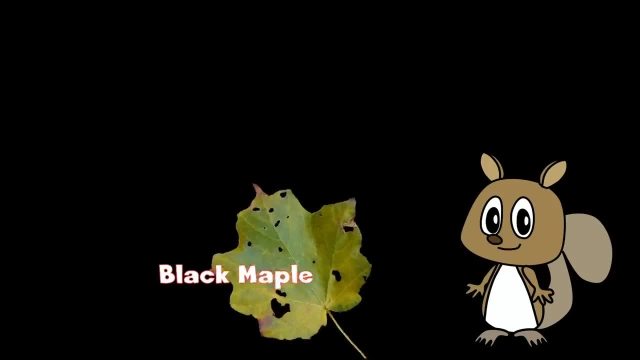 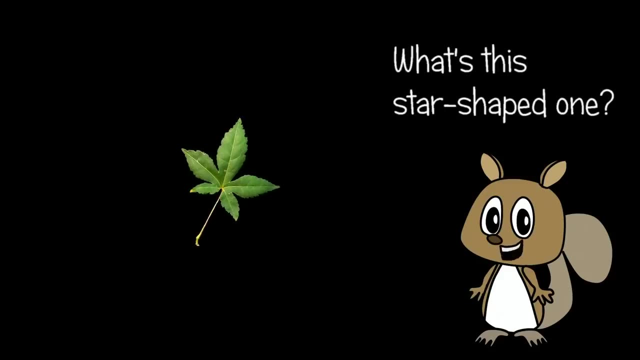 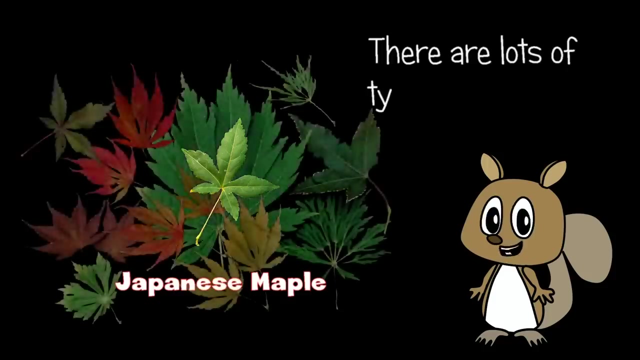 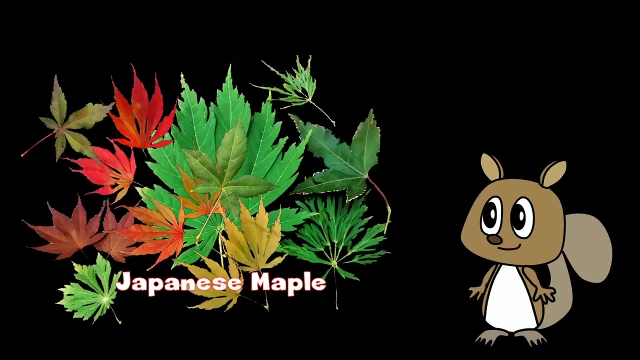 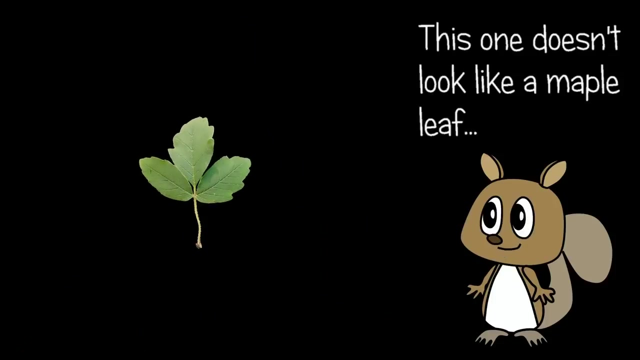 It's a black maple leaf. What's this star-shaped one? It's a Japanese maple leaf. There are lots of types of Japanese maples. you can often find them in gardens. They're beautiful. This one doesn't look like a maple leaf, But it is. It's called paper bark maple. 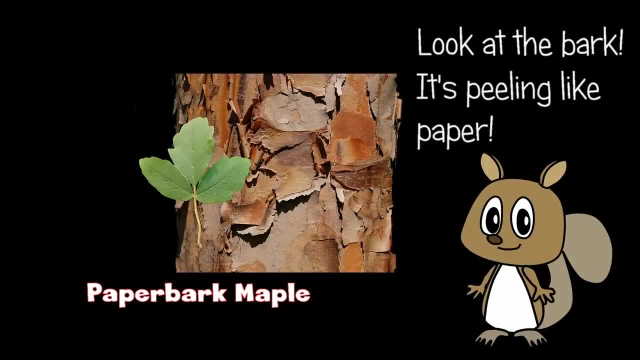 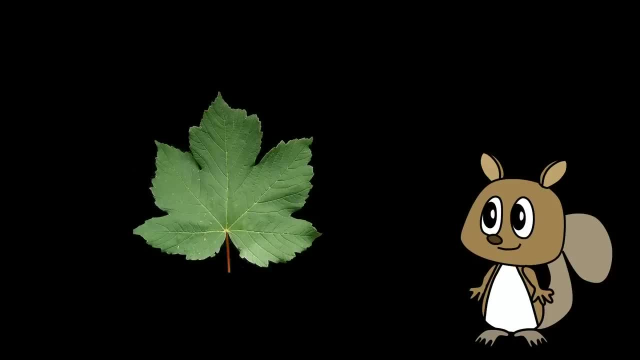 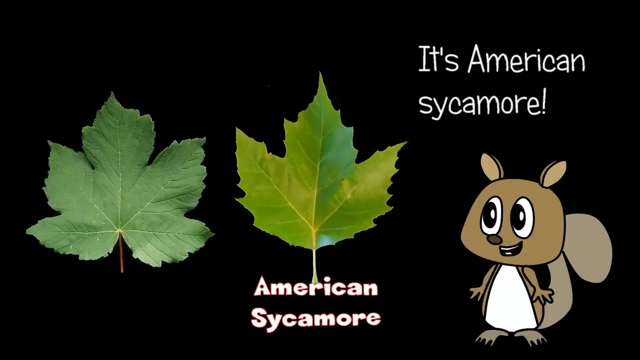 Look at the bark. It's peeling like paper. Wow, this one's big. It has five wide lobes. This is a sycamore maple leaf. Another big one, It's American sycamore. Both of them have sycamore in their names. 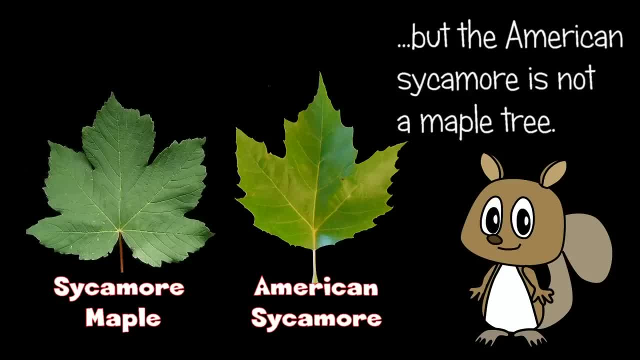 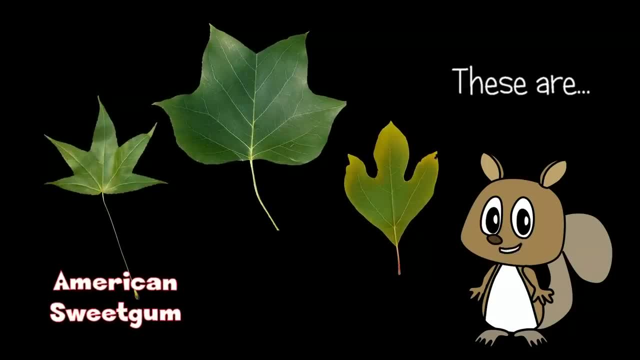 But the American sycamore is not a maple tree. These are American sweetgum, tulip tree and sassafras. These are American sweetgum, tulip tree and sassafras. These are American sweetgum, tulip tree and sassafras. 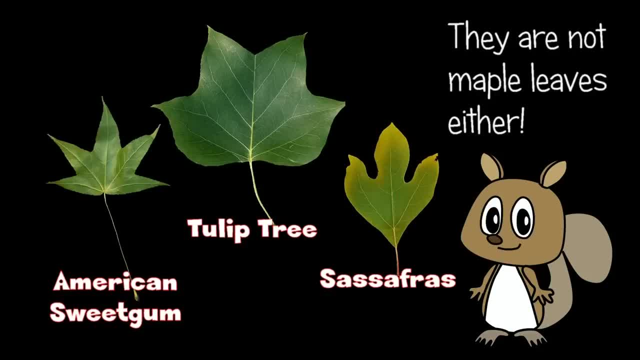 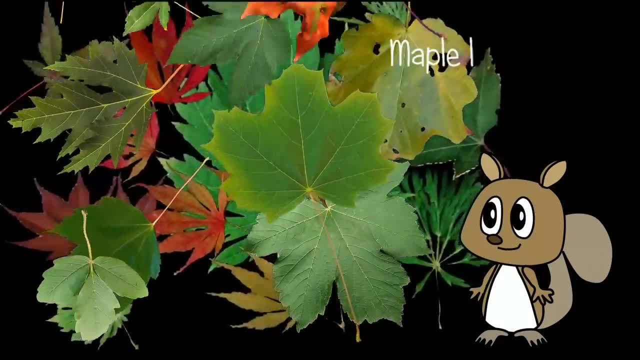 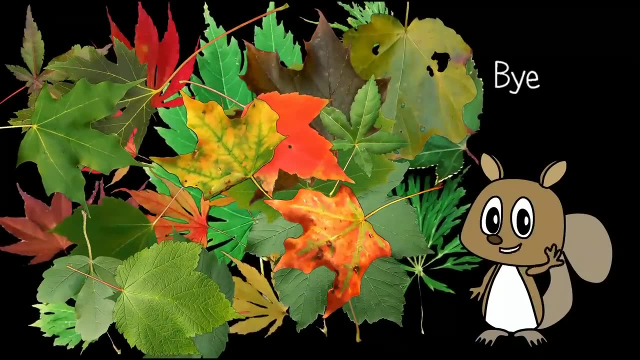 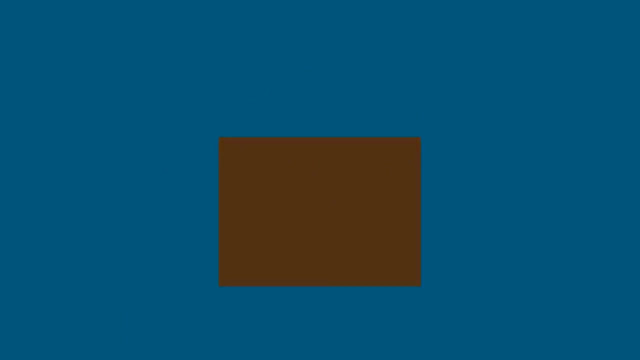 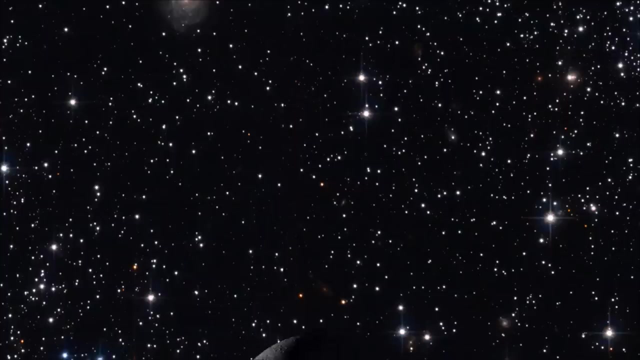 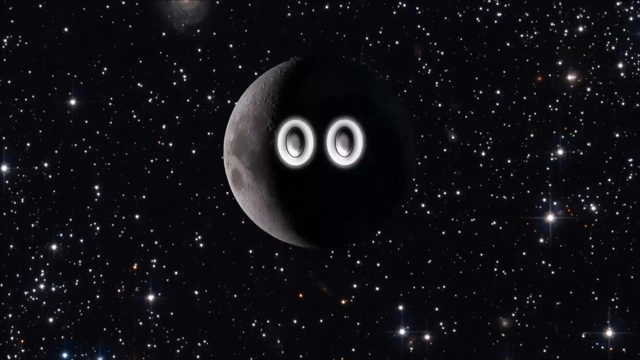 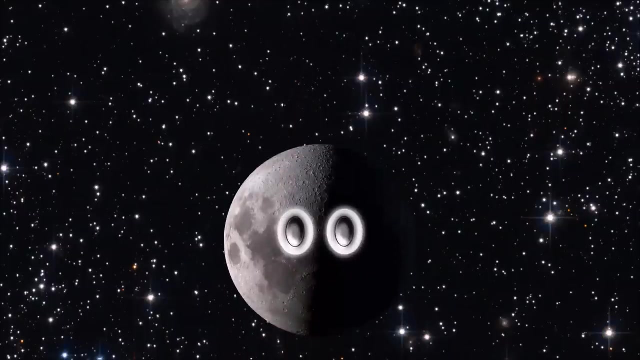 They are not maple leaves either. Maple leaves are beautiful and fun. Thanks for watching. Bye-bye. Keep watching for more Phases of the Moon. Bye, bye. Phases of the Moon from the Southern Hemisphere. Phases of the Moon from the Southern Hemisphere sphere: waxing crescent. 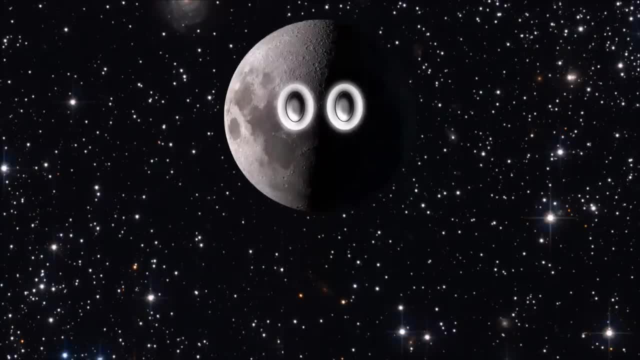 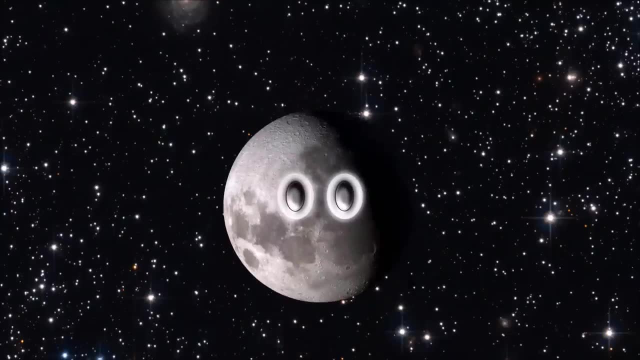 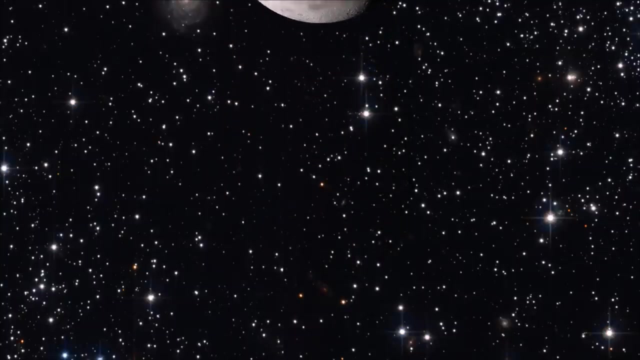 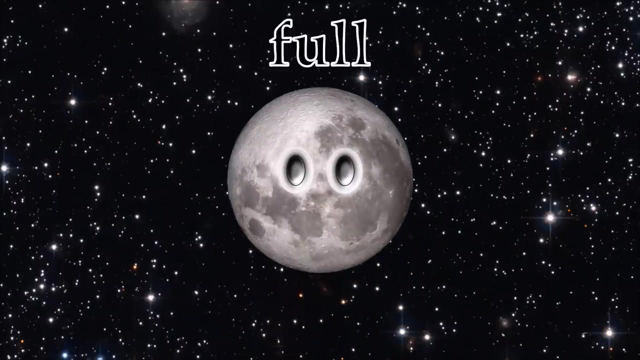 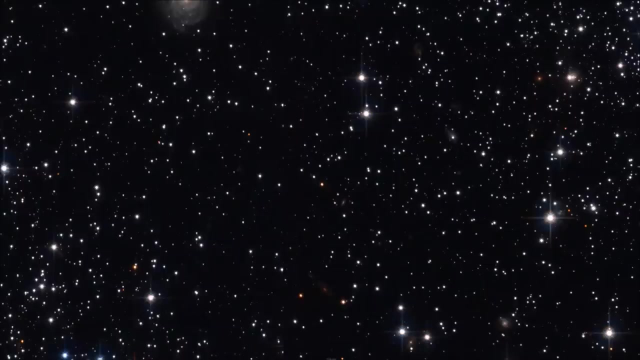 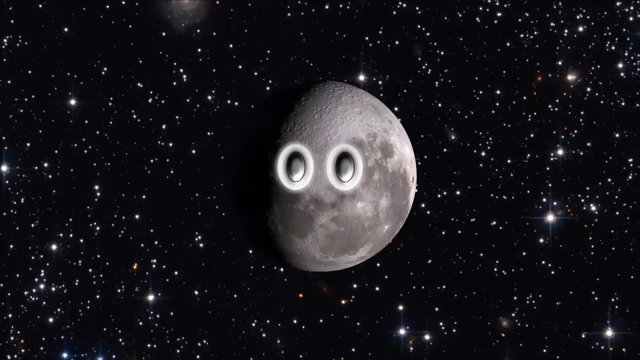 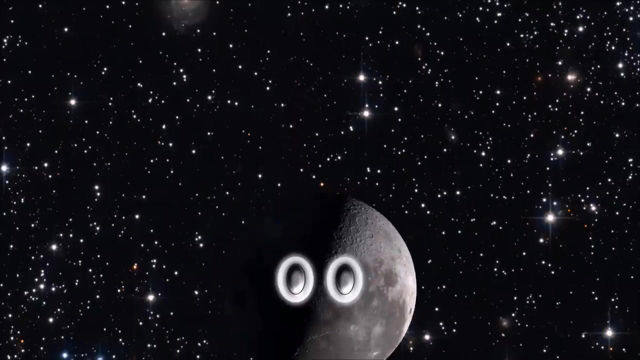 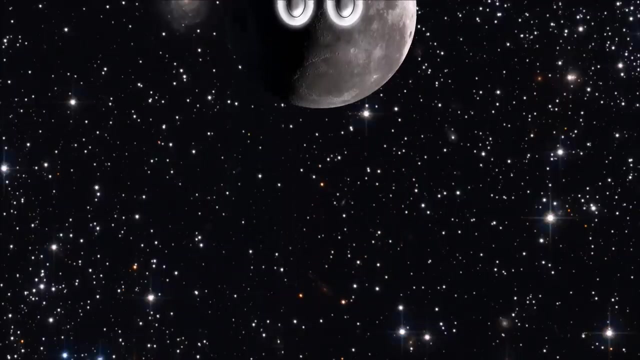 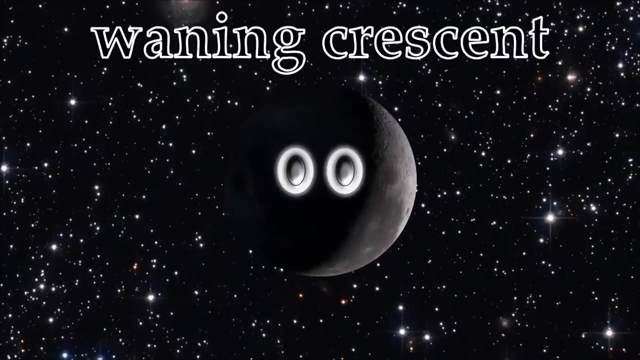 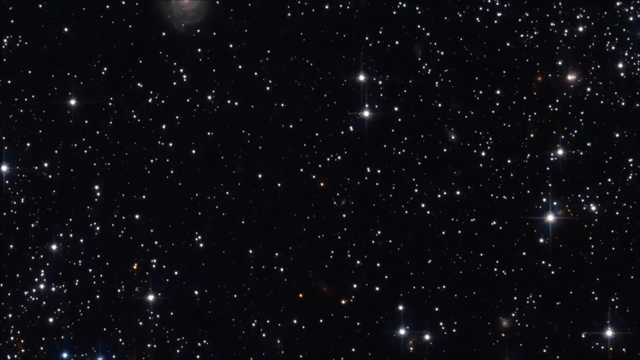 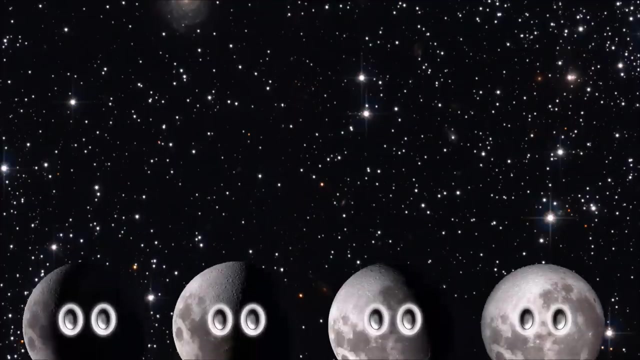 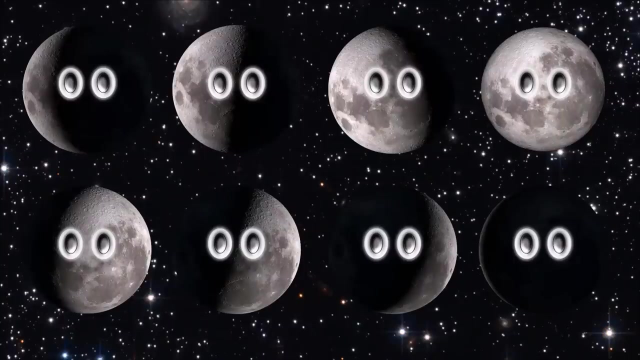 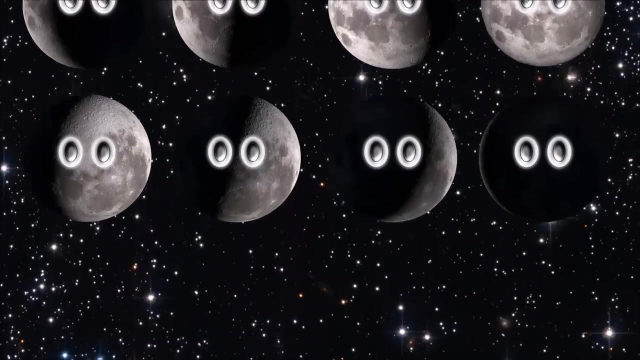 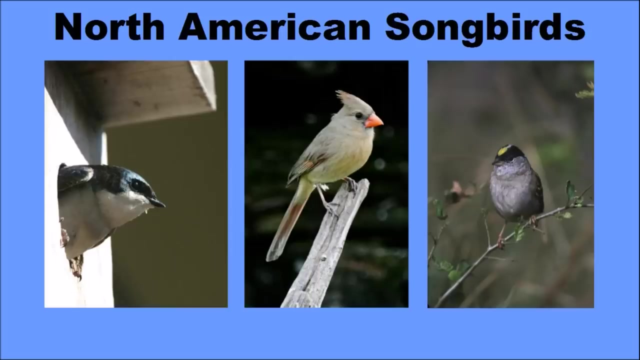 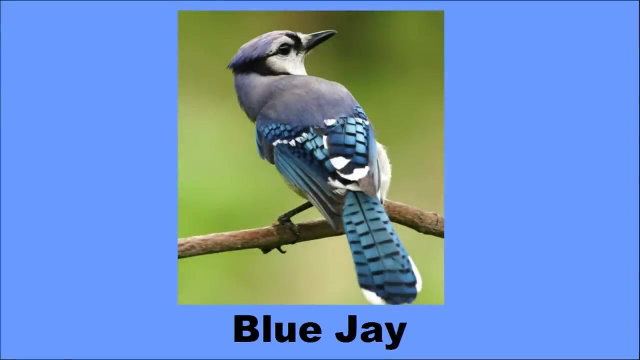 first quarter waxing gibbous, full first quarter waxing. first quarter: waning gibbous. third quarter, waning gibbous. third quarter, waning gibbous, waning, crescent, new. Next up is North American songbirds, North American songbirds, Blue jay. 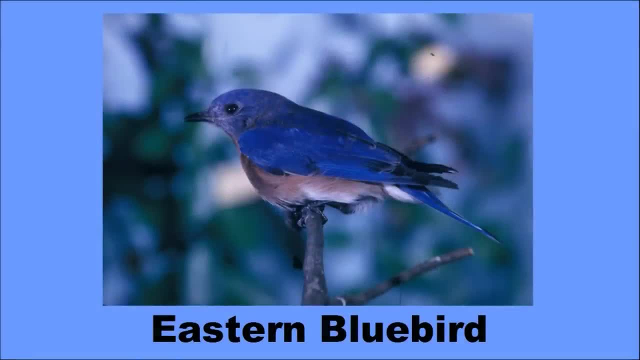 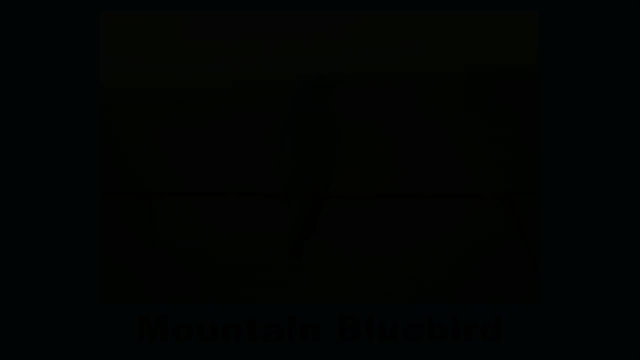 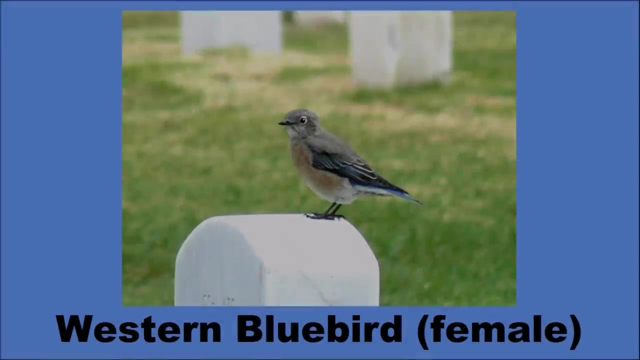 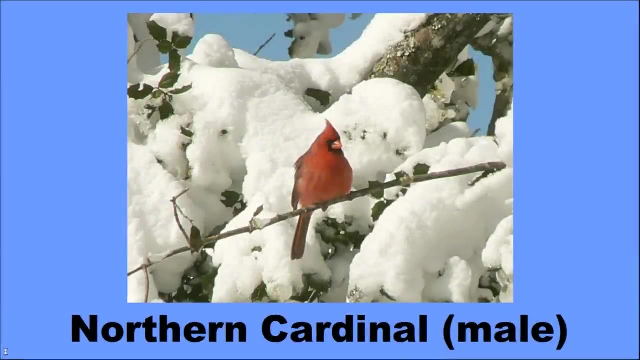 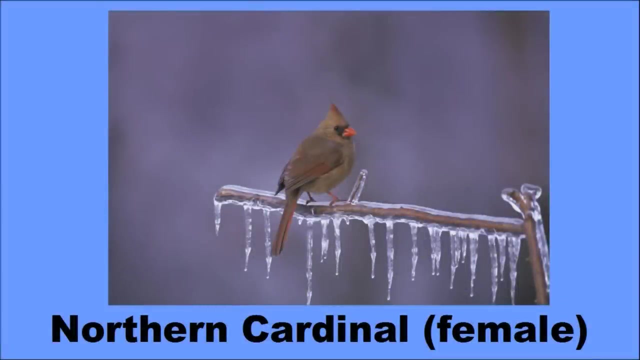 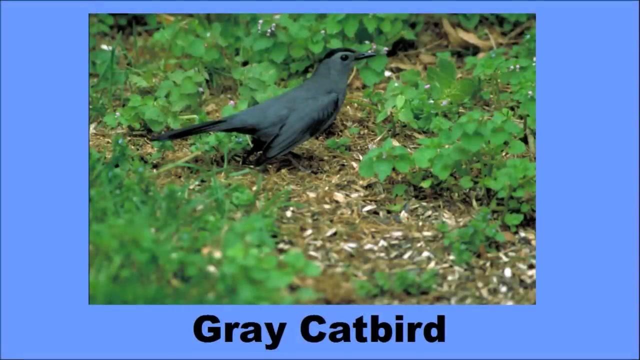 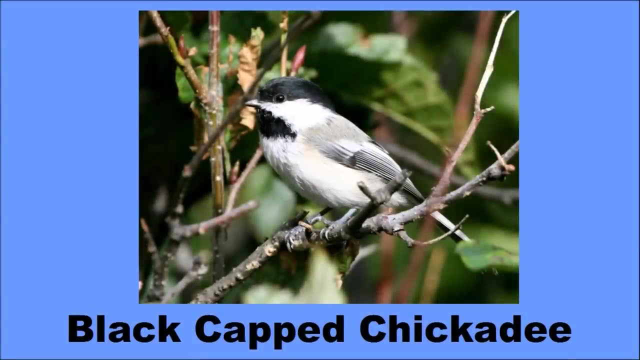 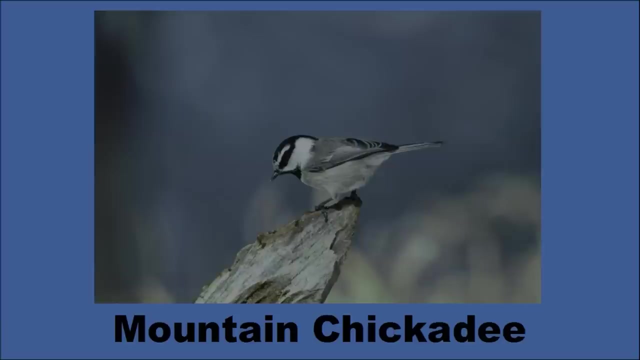 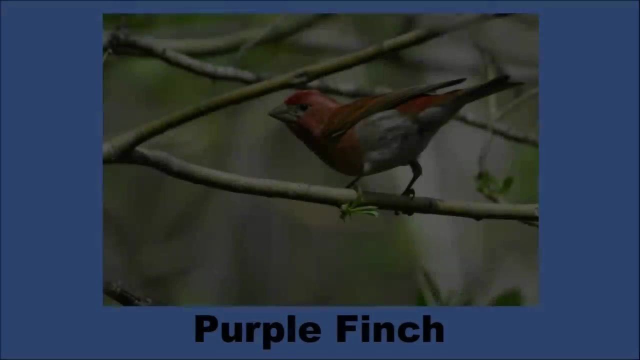 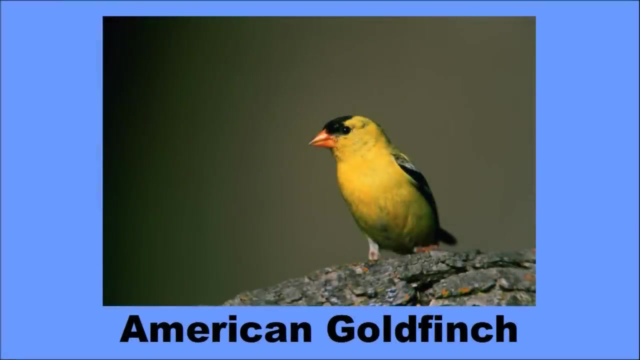 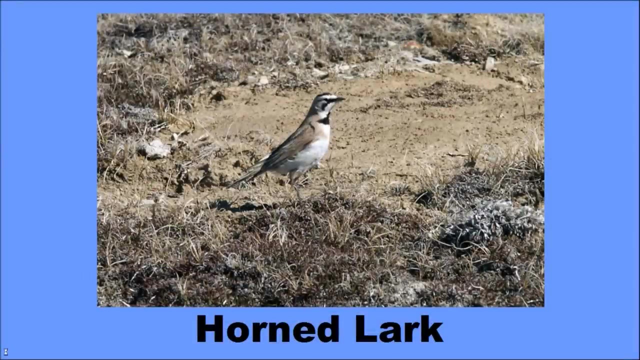 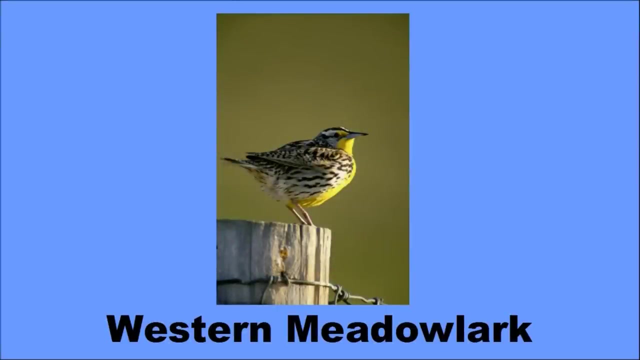 Eastern bluebird Mountain bluebird. Western bluebird male. Western bluebird female. Northern cardinal. male Northern cardinal female. Gray catbird, Black-capped chickadee Mountain, chickadee House, finch, Purple finch, American goldfinch, Horned lark, Western meadowlark. 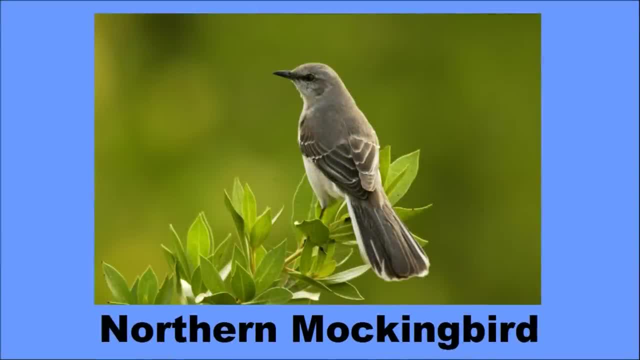 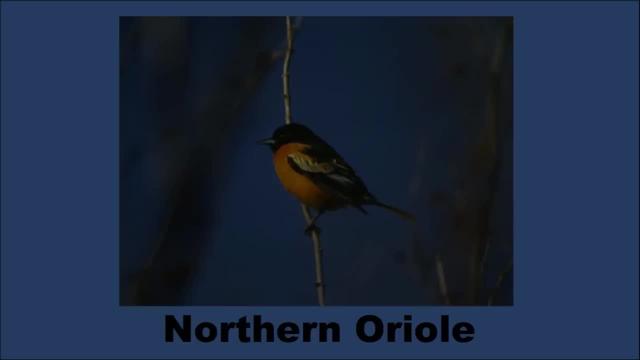 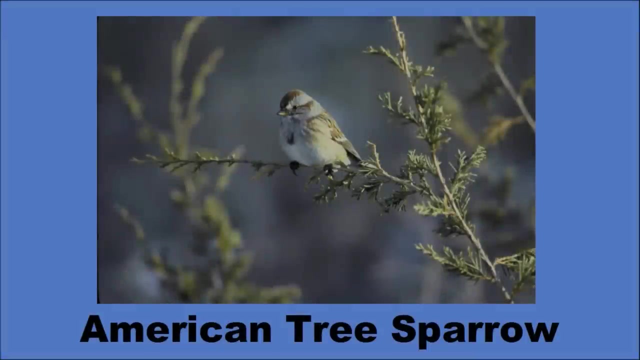 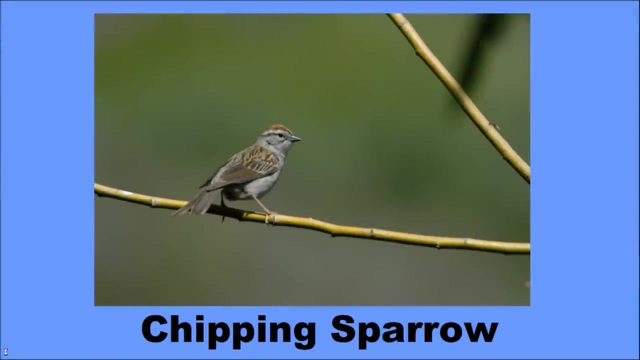 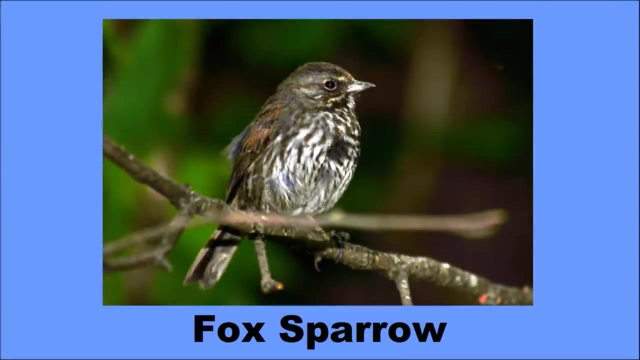 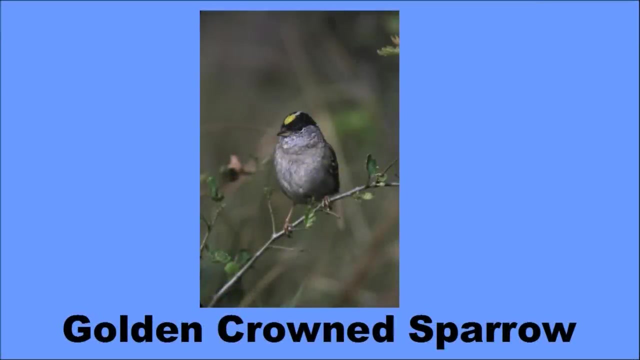 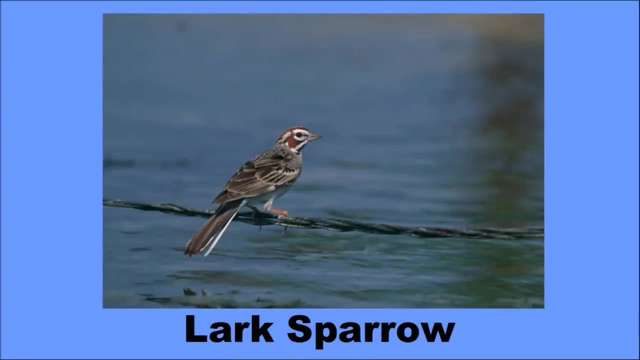 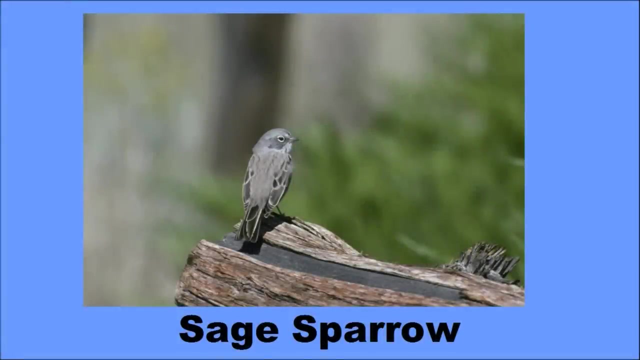 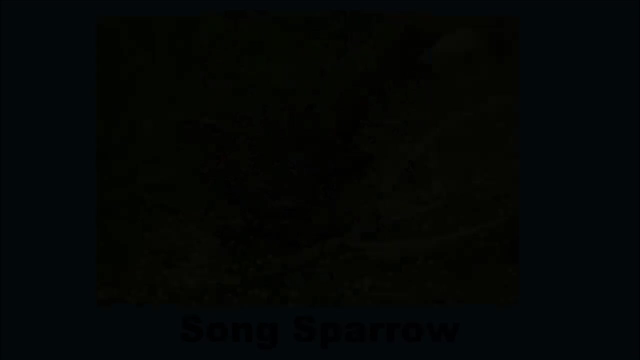 Northern mockingbird, Northern oriole, American robin, American robin, American tree sparrow, Chipping, sparrow, Chipping. sparrow Fox, sparrow Fox, sparrow, Golden-crowned sparrow, Golden-crowned sparrow. Lark, sparrow, Sage, sparrow, Savannah, sparrow Song sparrow.